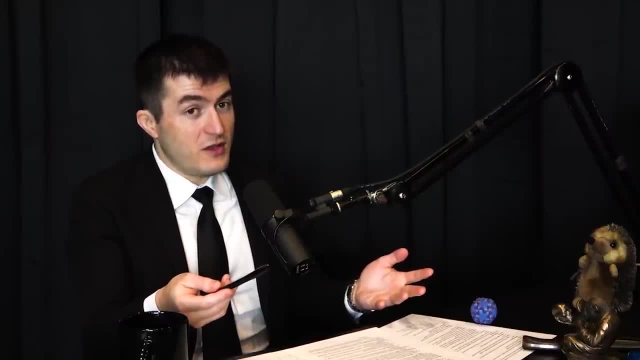 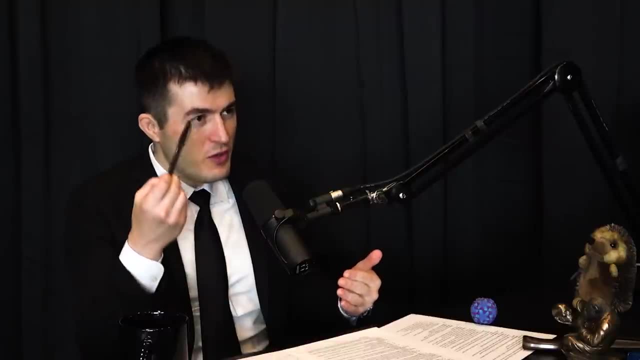 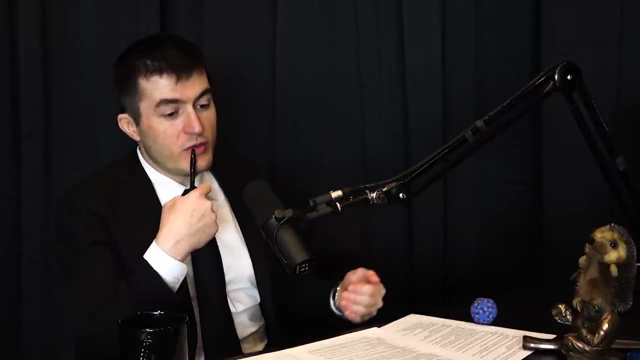 and Psycorp is the knowledge. Have you ever considered just like throwing away the code base and starting from scratch- Not really throwing away but sort of moving it to like throwing away that technical debt, starting with a more updated programming language? 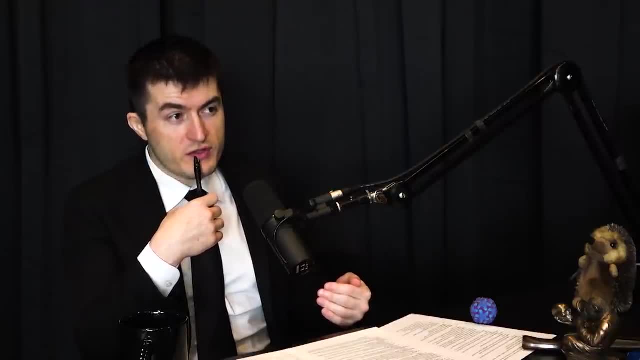 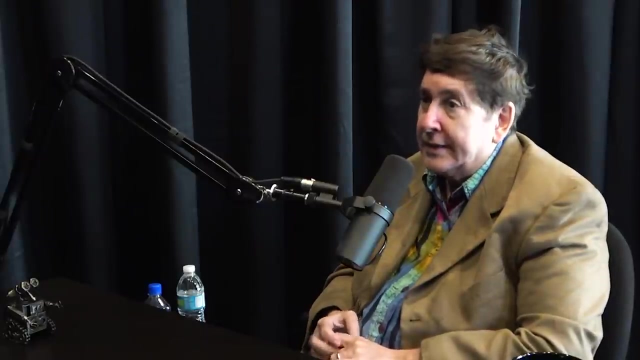 Is that throwing away a lot of value or no, Like what's your sense? How much of the value is in the silly software engineering aspect And how much of the value is in the knowledge? So development of programs in Lisp proceeds. I think somewhere between a thousand and. 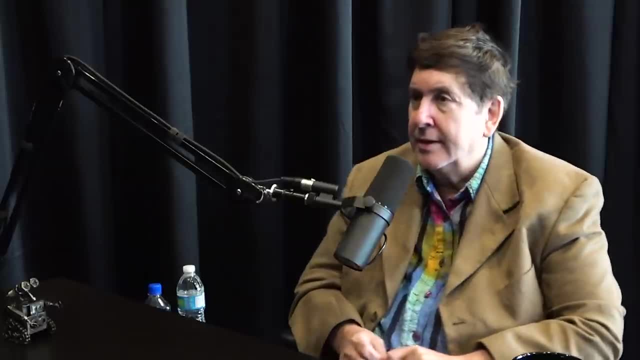 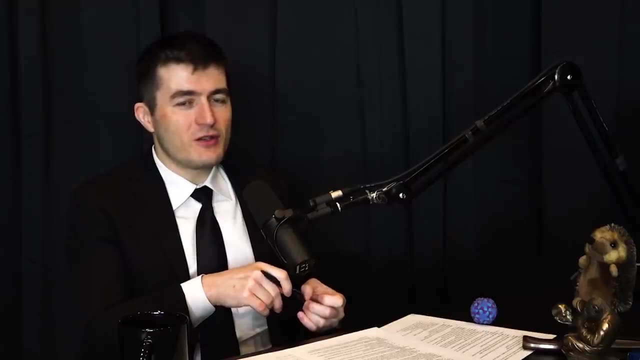 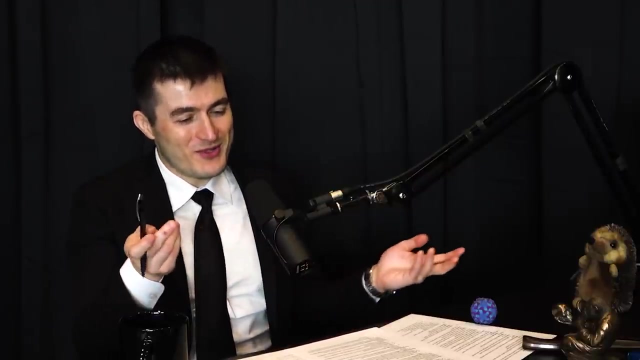 50,000 times faster than development in any of what you're calling modern or improved computer languages. Well, there's. there's other functional languages, like you know: Clojure and all that there there's. but I mean, I'm with you, I like Lisp. I just wonder how many great programmers there are. 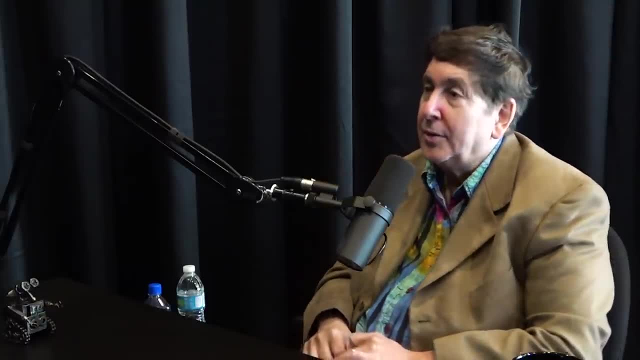 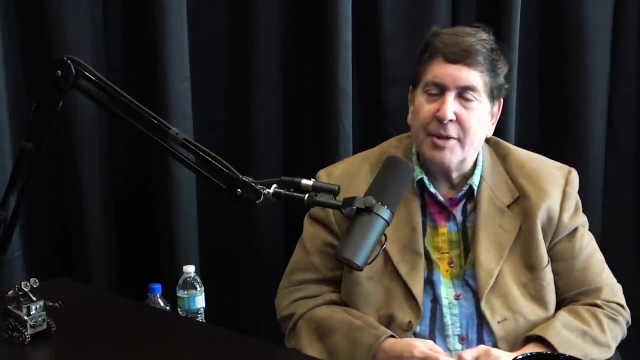 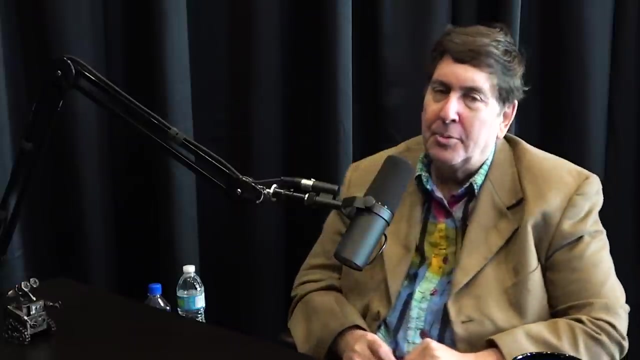 There's still like Yes. So so it is true, when a new inference programmer comes on board, they need to learn some of Lisp, And in fact we have a subset of Lisp, which we call cleverly sub L, which is really all they need to learn, And so the programming actually goes on in sub L, not in. 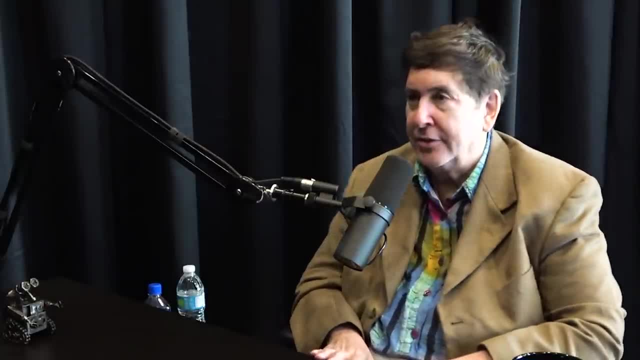 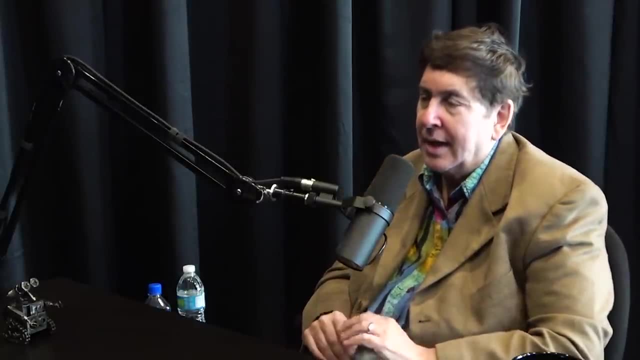 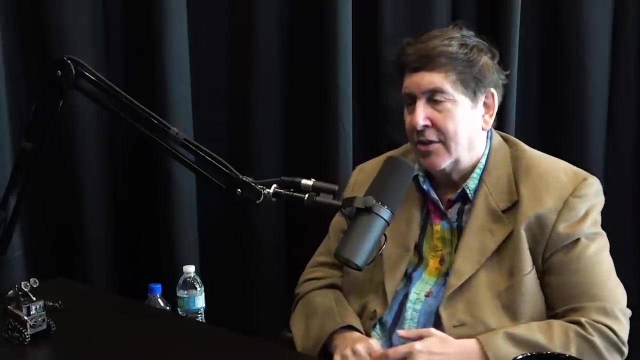 full Lisp, And so it does not take programmers very long at all to learn sub L, And that's something which can then be translated efficiently into Java, And for some of our programmers who are doing, say, user interface work, then they never have to even learn sub L, they just have to learn. 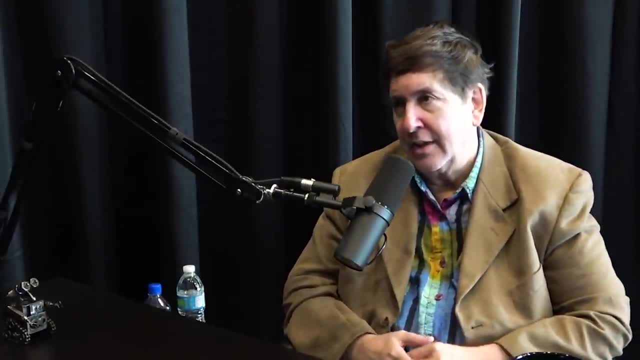 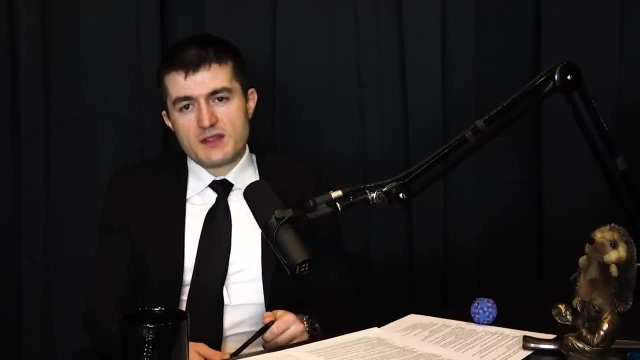 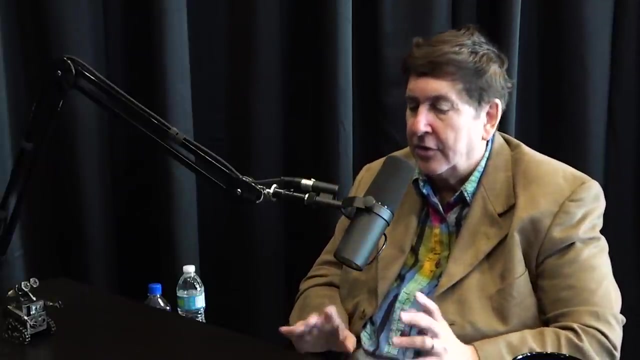 API's into the basic psych engine, So you're not necessarily feeling the burden of like it's extremely efficient, there's that's not a problem to solve, Right? The other thing is remember that we're talking about hiring programmers to do inference, who are programmers interested in effectively automatic theorem proving, And so 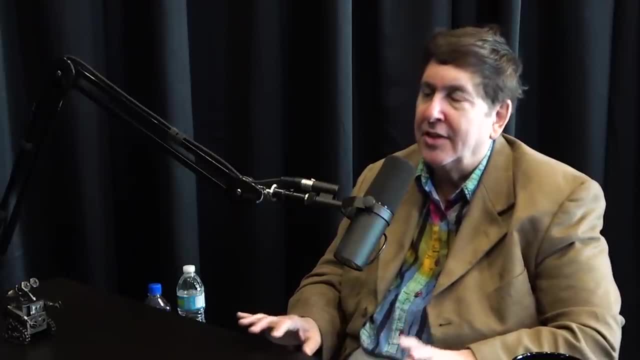 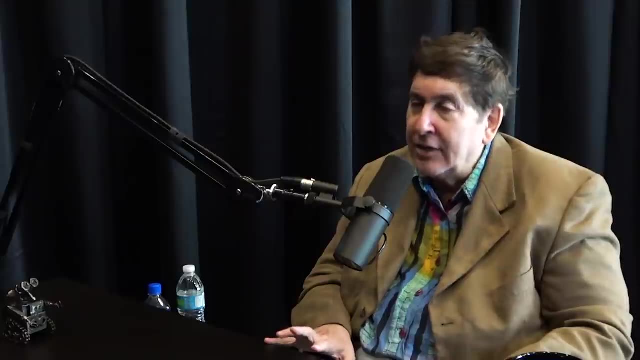 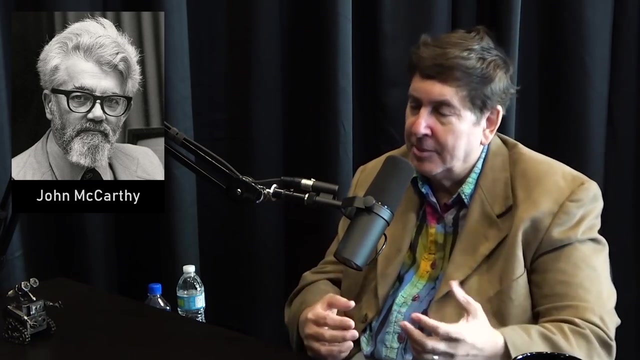 those are people already predisposed to representing things in logic and so on. And Lisp really was the programming language based on logic that John McCarthy and others who developed it basically took the formalisms that Alonzo Church and other philosophers, other logicians, had come up with. 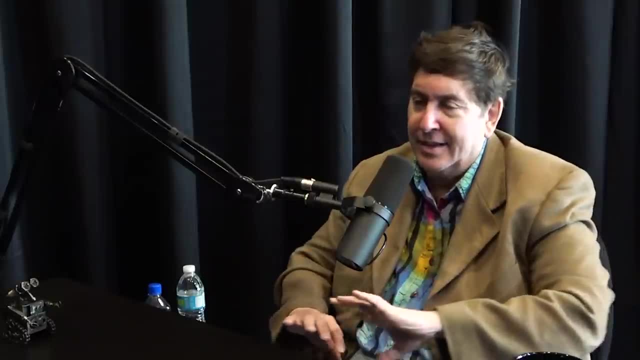 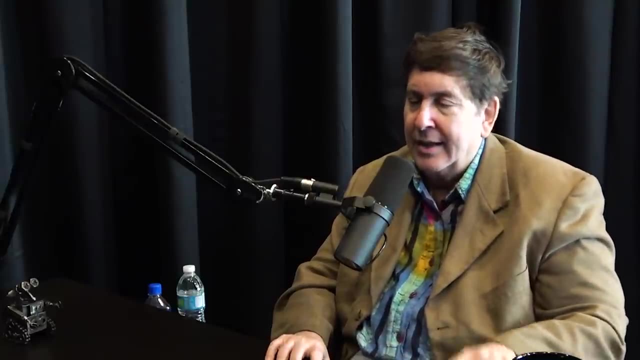 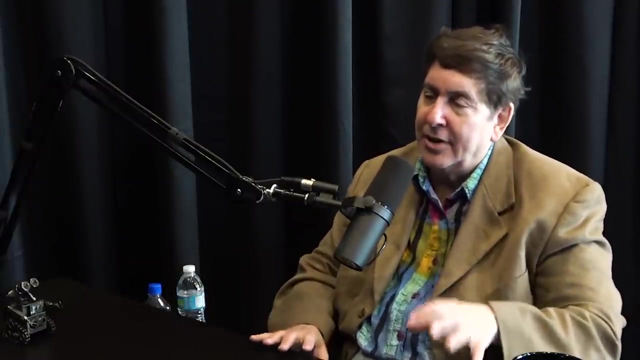 and basically said: can we basically make a programming language which is effectively logic? And so, since we're talking about reasoning in expressions written in this logical, epistemological language and we're doing operations which are effectively like theorem proving, type operations and so on, let's see if you can follow the basics of what I was talking about. So ask this liquid Mark, because we've discussed sort of we're not even in themes of, but we don't just go with it. So at least you could answer the question, Melanie. Ah, all right. 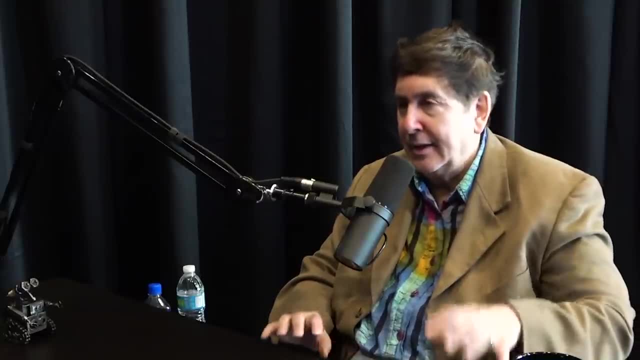 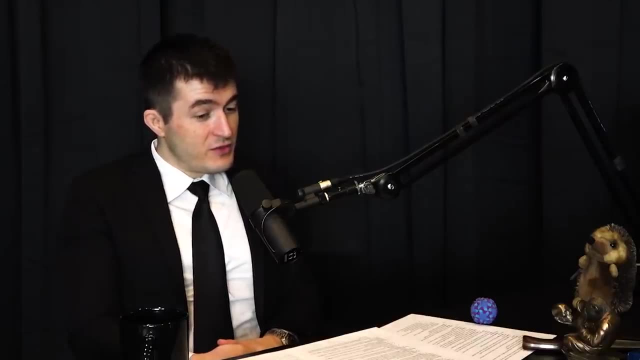 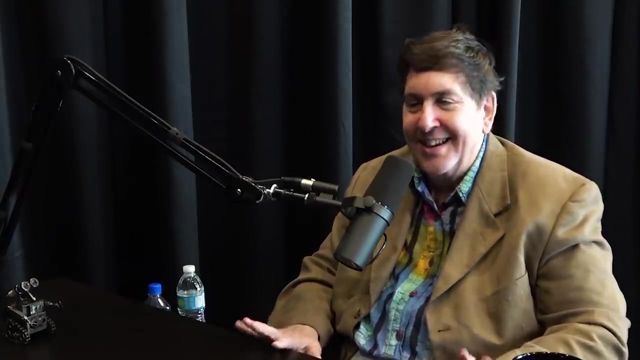 is a natural impedance match between lisp and the- the knowledge, the way it's represented. so i guess you could say it's a perfectly logical language to use. oh yes, okay, i'm sorry, i'll even let you get away with that. okay, i know i like that, so i'll probably use that in the future without. 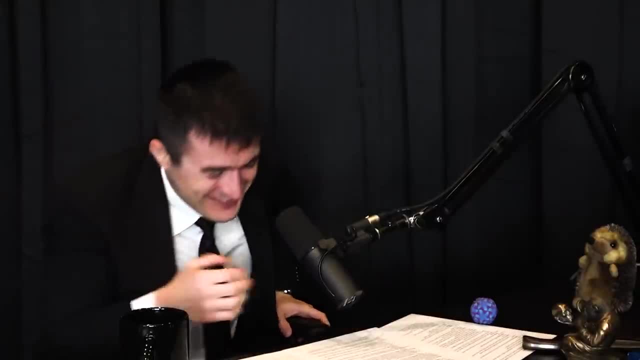 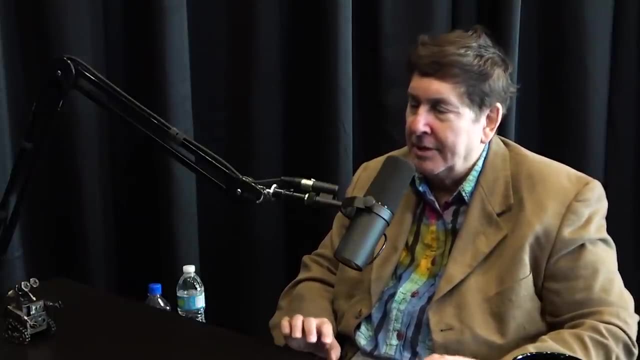 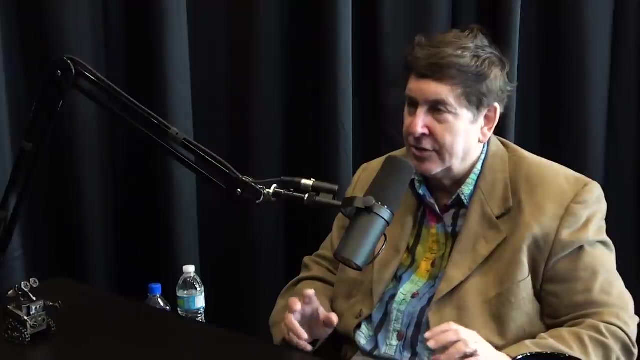 without credit. without credit, but no, i think. i think the uh, the. the point is that the, the language you program in, isn't really that important. it's more that you have to be able to think in terms of, for instance, creating new helpful hl modules and how they'll work with. 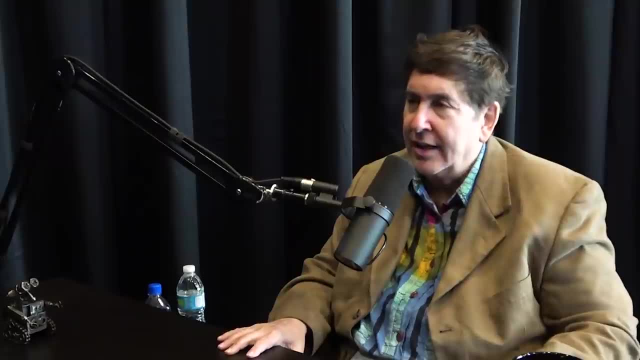 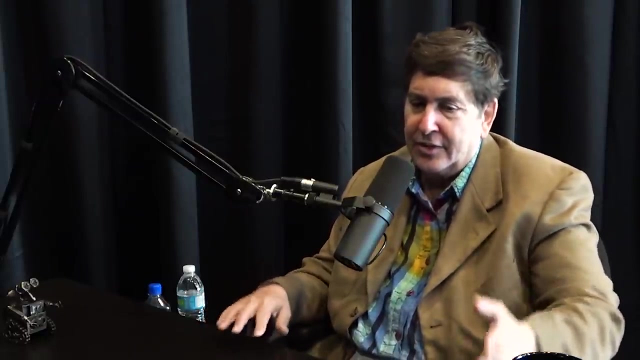 each other and looking at things that are taking a long time and coming up with new specialized data structures that will make this efficient. so let me just give you one very simple example, which is when you have a transitive relation like larger than this is larger than that which is larger than that which is larger than that. so the first 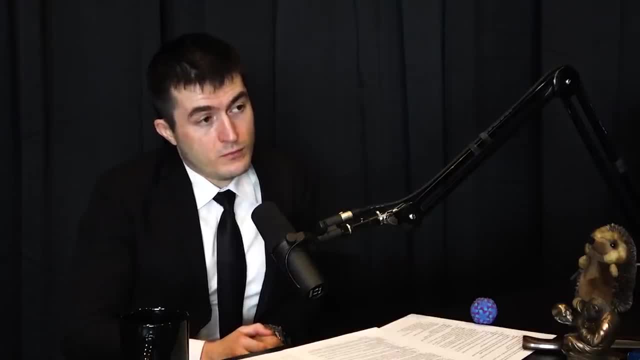 thing must be larger than the. the last thing whenever you have a transitive relation. if you're not careful, if i ask whether this thing over here is larger than the thing over here, i'll have to do some kind of graph walk or theorem proving. that might involve like 5 or 10 or 20. 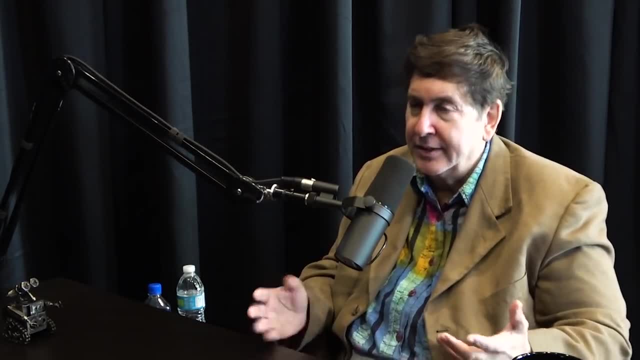 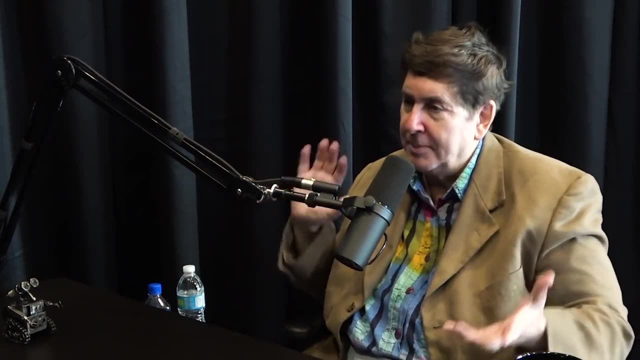 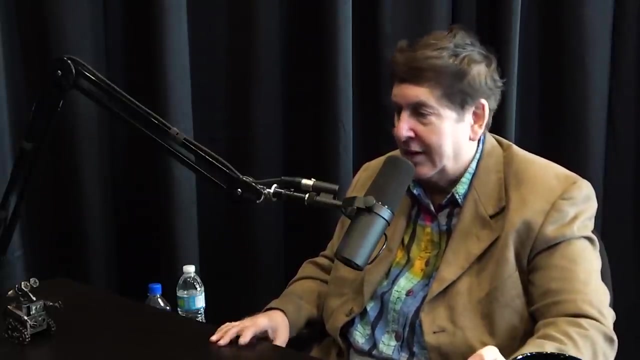 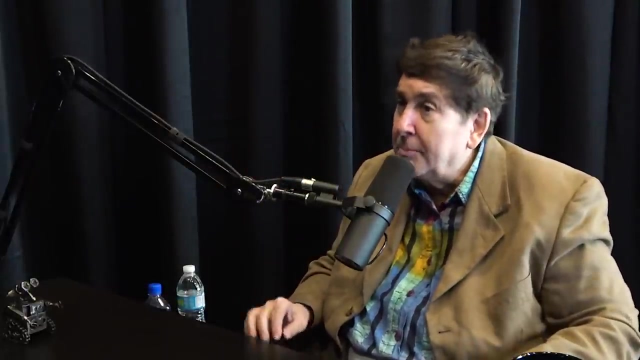 or 30 steps. but if you store redundantly, store the transitive closure, the cleanly star of that transitive relation, you have this big table but you can always guarantee that in one single step. you can just look up whether this is larger than that. and so we. there are lots of cases where storage is cheap.